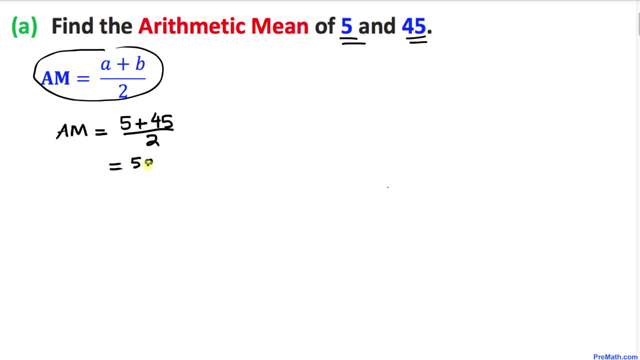 it by 2.. So we are going to get 50 divided by 2.. So that means our arithmetic mean turns out to be simply 25.. So that's the arithmetic mean of these two numbers, 5 and 45, turns out to be a 25.. 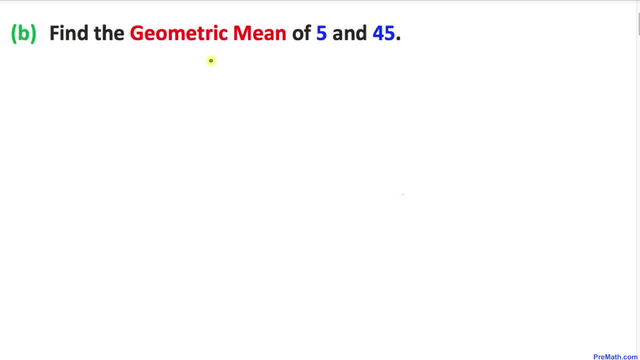 And now let's talk about the geometric mean mean. and here's the geometric mean description. the geometric mean works when the data is in a multiplicative relationship. that means we are dealing with the multiplication of the numbers. the geometric mean is used when the data is not linear. and here's the geometric mean formula. 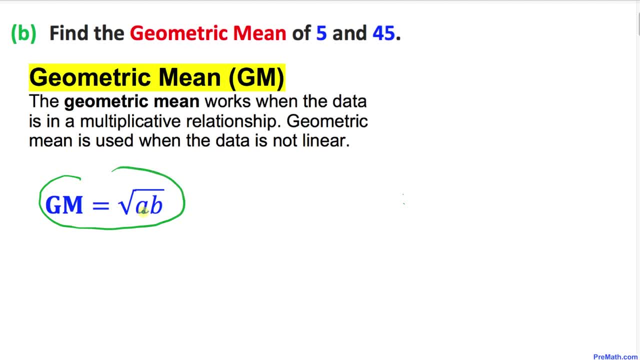 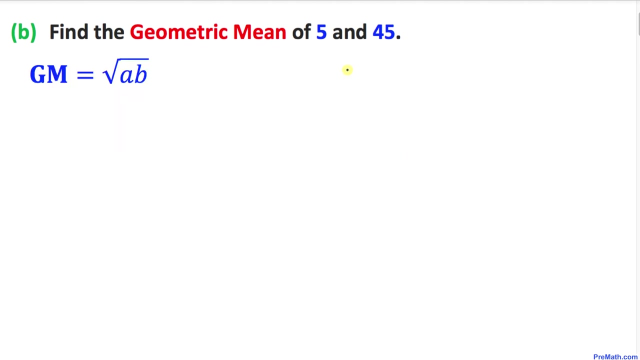 geometric mean equal to the square root of two numbers, a and b. and here's another formula of geometric mean as well. this is, in terms of proportion, a over x, equal to x over b, and i will show you both methods in this given example. now let's go ahead and calculate the geometric 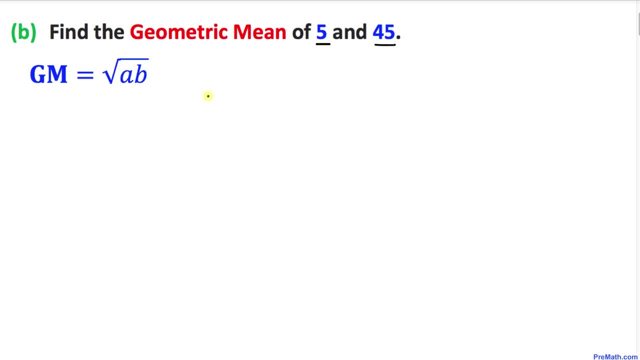 mean of these two numbers, five and 45. and here's our formula. let's go ahead and fill in the blanks. so geometric mean is going to be the square root of a. in our case is five times. the second number is 45. let's go ahead and multiply. 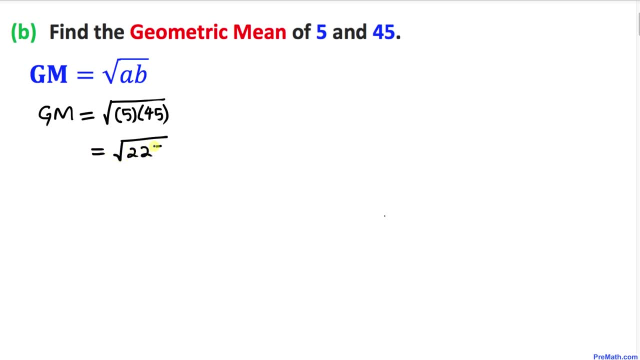 them out. so that is going to give us 225. the square root of 225 is 15, so our geometric mean of these two numbers turns out to be 15.. now let me show you this proportion formula to find that this geometric mean. and just keep in your mind that x represents the geometric mean of 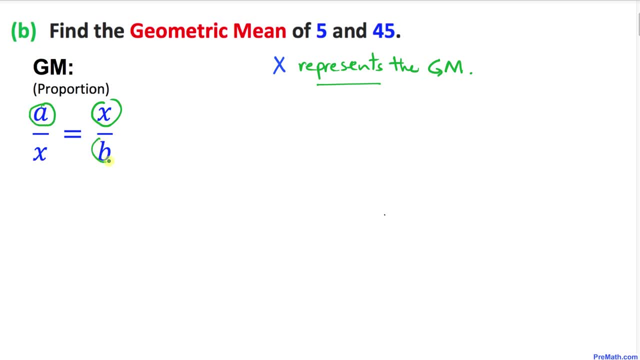 these two numbers, a and b. now let's go ahead and fill in the blanks wherever we see a. a, in our case, is five and b is 45. so let's go ahead and fill in the blanks and we will see that x is 45 and b is 45. 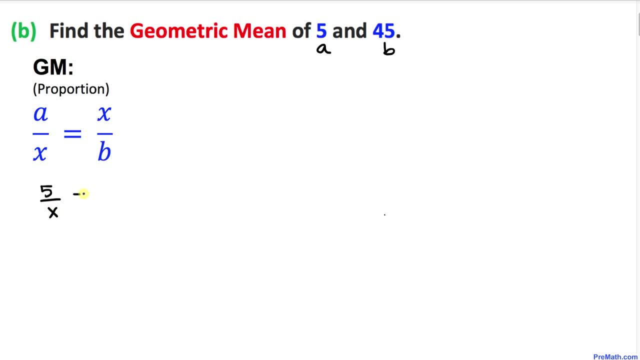 let's go ahead and write down: five over x, equal to x over 45. let's go ahead and cross multiply. when we cross multiply, we are going to get five times 45 is 225, x times x is x square. let's take the square root on both side to undo this square, so this square and 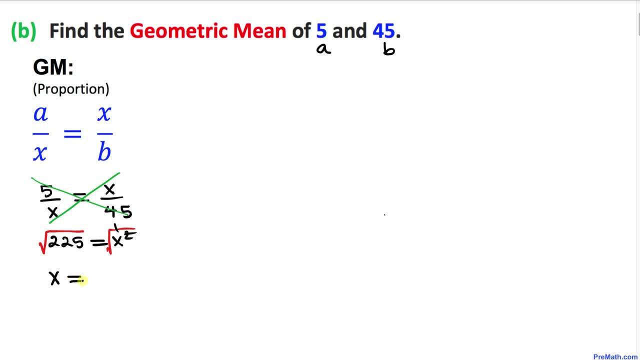 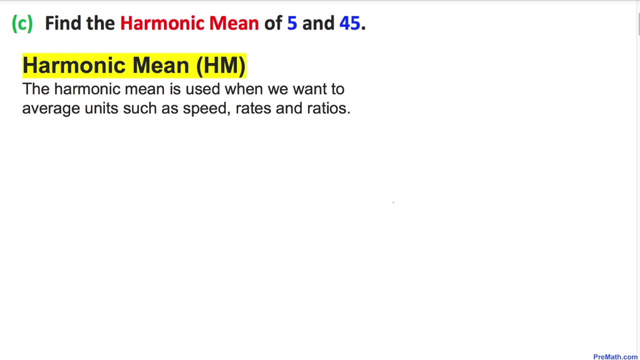 square root. this is gone, so our x value turns out to be simply 15, and this is our geometric means. so that's the geometric mean of 5, and 45 turns out to be 15. and now let's talk about the harmonic mean, and here's our harmonic mean description. the harmonic mean is used when we want to find: 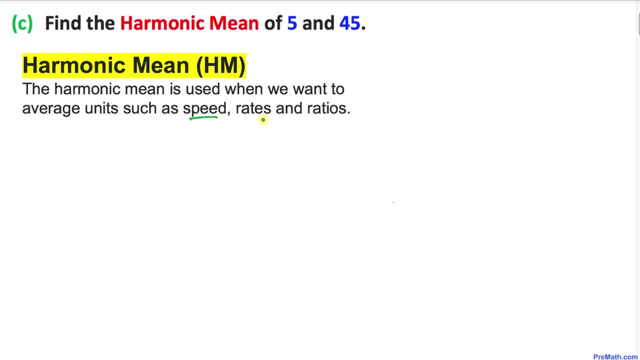 the average of things like speed rates are ratios. now let me give you one good example. my speed on the freeway was 60 miles per hour and the speed inside the city was 30 miles per hour. what is my average speed? and here i have just calculated the average speed. my question is: is this the correct way? question mark: oh, this is. 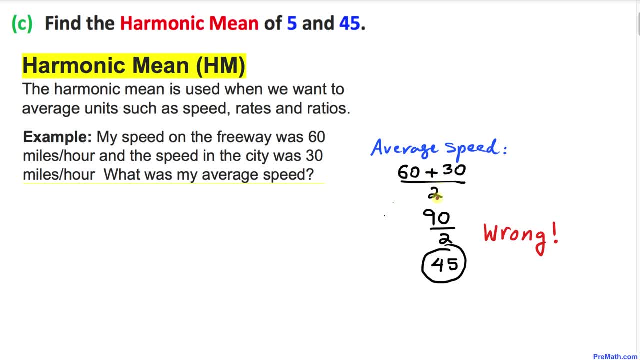 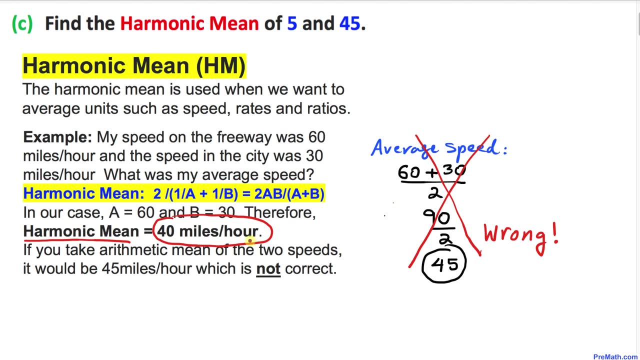 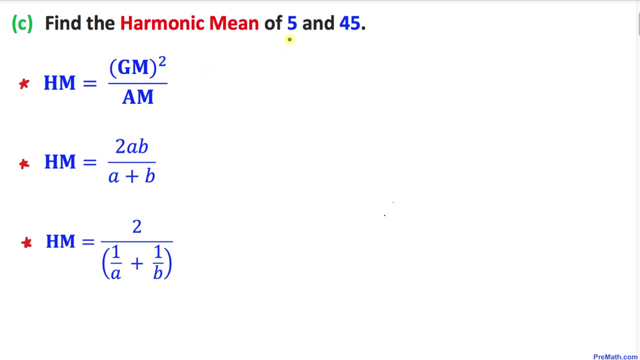 the wrong method. we cannot just simply add these two numbers and divide by two and we get the answer. and the correct answer is supposed to be 40 miles per hour. we will be calculating the harmonic mean, and i will show you this method little bit later. and here are the three different formulas to calculate the harmonic mean of these. 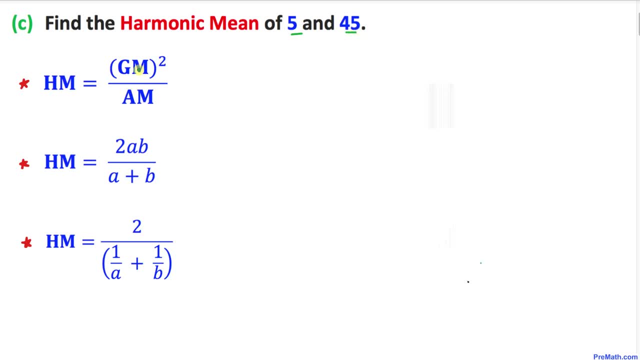 two numbers. the first one is gm, means the geometric mean squared divided by arithmetic mean. the second one is 2ab divided by a plus b. and the third one is 2 divided by 1 over a plus 1 over b, and i will show you these three different methods in our this. 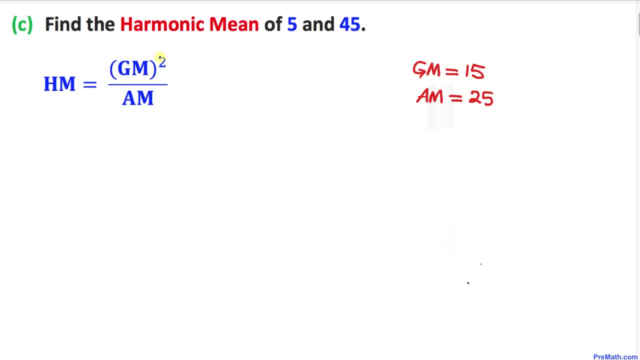 example. and now let me show you the first formula to calculate the harmonic mean of these two numbers, 5 and 45. and here's our formula: gm squared divided by am. we figured out our geometric mean, gm 15, our previous step- and arithmetic mean as 25 as well, so let's go ahead and fill in the blanks. 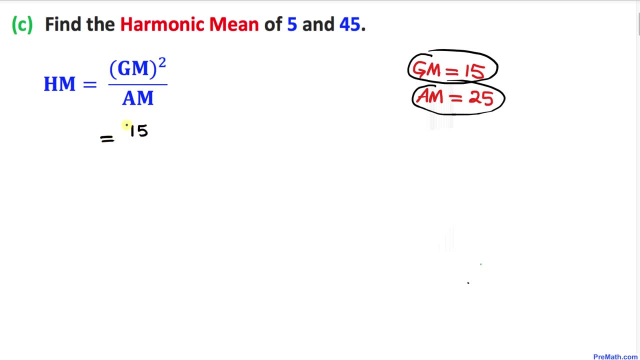 so gm is 15, and then square divided by am is 25. let's go ahead and simplify: 15 squared is 225 divided by 25, that is, we divide that thing. our harmonic means hm turns out to be simply 9, and let's go ahead and use the second formula now: 2 times a, b divided by a plus b, in our case. 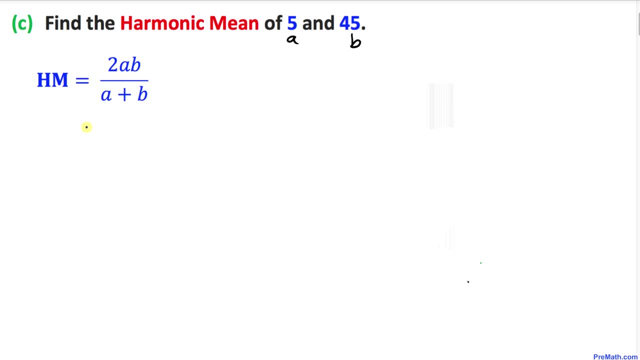 a is 5 and b is 45. let's fill in the blanks. so 2 times 5 times 45, divided by 5 plus 45, and here if we multiply the numerator numbers, we get 450 divided by denominator 50. and if we simplify, our harmonic mean turns out to be 9. and now let me show you this third formula. 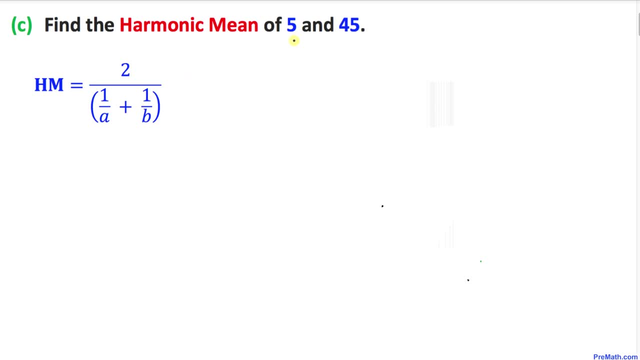 how to apply this one, and here our a is 5 and b is 45. let's go ahead and fill in the blanks. so 2 divided by 1 over a, in our case, is 5 plus 1 over 45. let's go ahead and simplify the denominator. 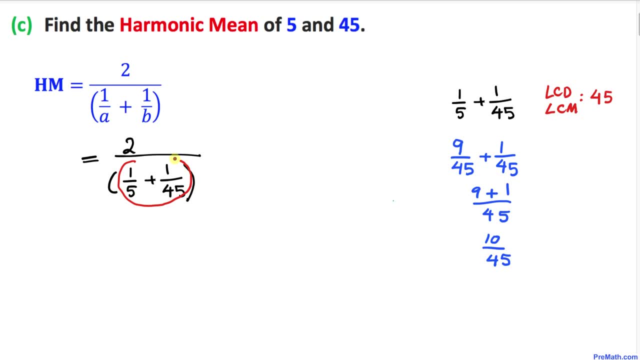 and here let's focus on this denominator part, these fractions i have just copied down over here. now let's add these two fractions. we know that our least common denominator, or sometime we call it least common multiple, is 45. we can make this one 45 by just multiplying and dividing by.